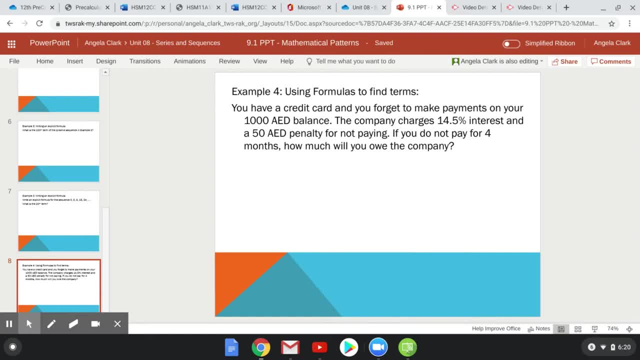 Alright, this is the last video of 9.1.. We're going to do a word problem writing a recursive formula. So you have a credit card and you forget to make your payment. on a $1,000 Durham balance, The company charges 14.5% interest and $50 Durham penalty for not paying. If you do not pay for four months, how much would you owe the company? 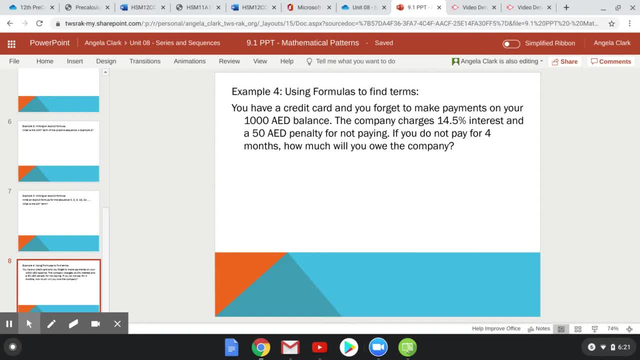 So we're going to write a recursive formula. So the first thing we need is what is a one going to be? Because, remember, with recursive we have to use the previous term to find the next term, So we have to know what a one is at the beginning. So a one is just going to be our initial balance right At the beginning, the first month before we've had a chance to make an interest. 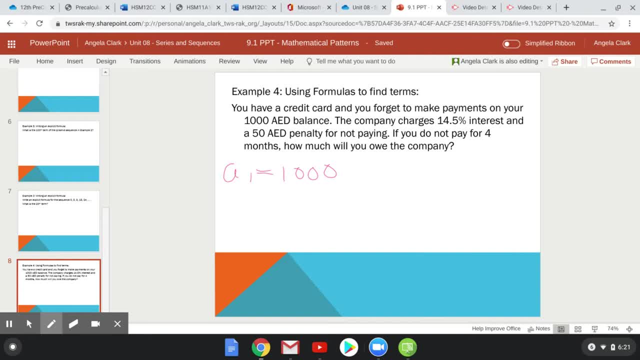 We're going to have $1,000 Durham, So that's going to be our first one. So then our formula. we need to figure out what a n is, And we know that it's going to have something to do with the previous one. We have to use the previous one to find the next one. So let's figure out how we're going to do that. And then to find- I want to just find what the next months would be right. I would take $1,000.. I would multiply that by my percentage to find my interest And then I would add the original amount on, So I'd get the interest plus the original amount. That would give me my new balance plus 50, right. 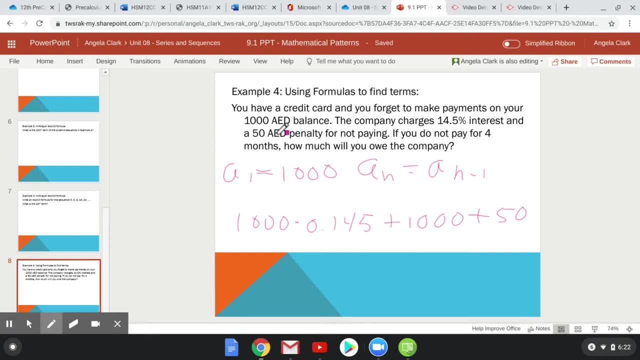 Because I need. I have to add that 50.. 50 Durham penalty fee. So I can simplify this down right To 1,000 times 0.145 plus 1 plus 50. So that's 1,000 times 1.145.. 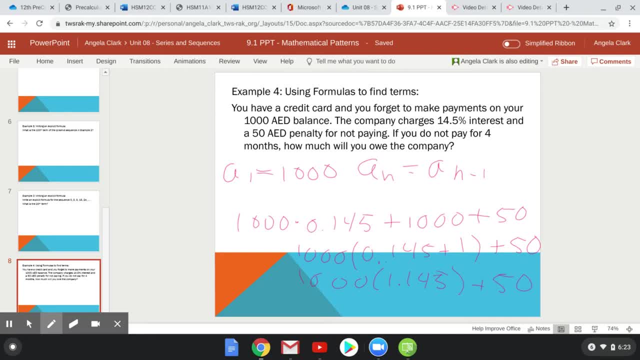 And this might be looking a little bit familiar. You might be saying, oh, I don't know. You might be saying, huh, that's kind of like what we were doing when we did exponential, except for we never had this extra thing that we were adding out here.